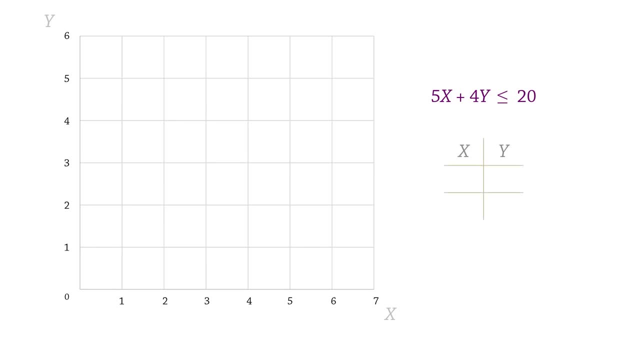 To draw the constraint line we only need two points, And we often use points where x and y are 0, since those are easy to calculate. So when x equals 0, here y is 5., And when y equals 0,, x is 4.. Joining those two points, we have the constraint line. Since this is a less than 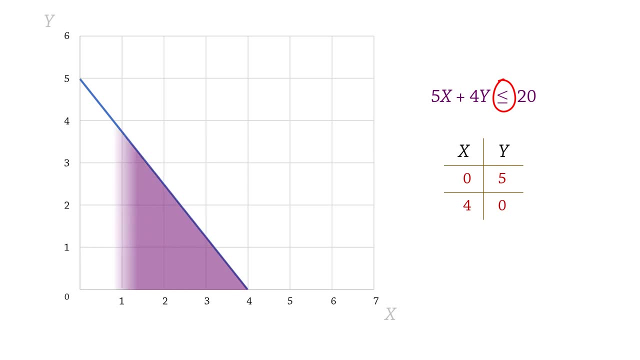 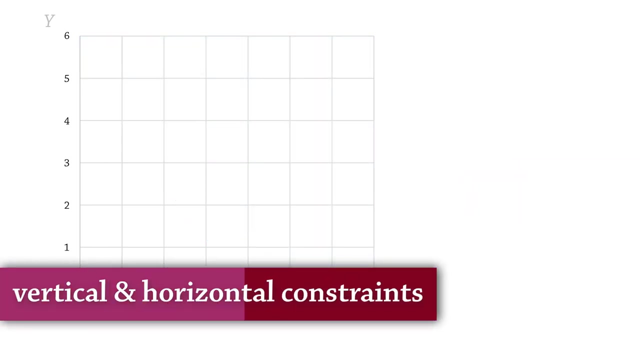 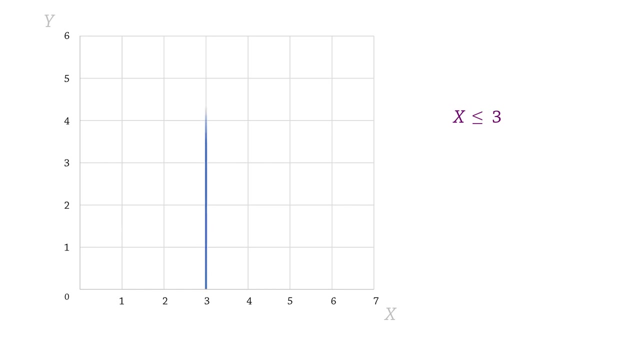 constraint, it will be satisfied below the line towards the origin here. And if it were a greater than constraint, it will be satisfied above the line away from the origin. Other basic constraints include those with vertical or horizontal lines. For example, to draw x less than or equal to 3, we start by drawing a line at x equals 3. 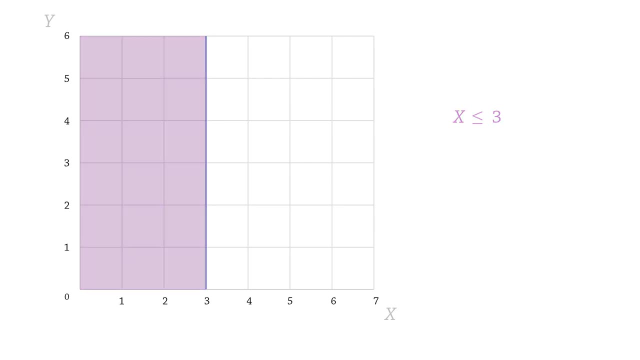 and shading the region to the left of it. And for x greater or equal to 4,, we shade the region to the right of 4.. Similarly, for y less than or equal to 2,, we shade the region below 2.. And for y greater or equal to 3,. 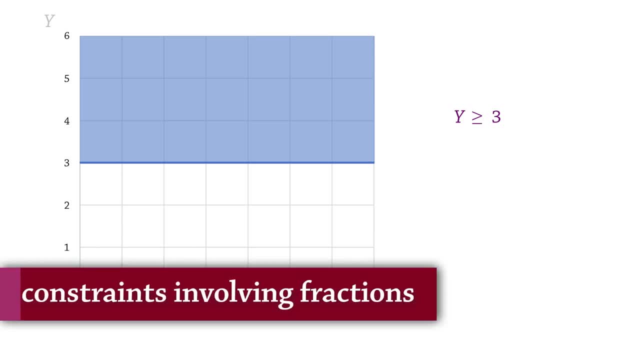 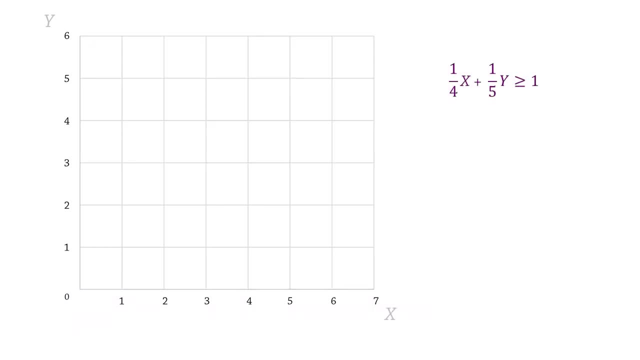 we shade the region below 2.. Sometimes our constraints involve fractions. Consider these constraints here, having fractions with denominators 4 and 5.. A good way to start is to clear the fractions. This can be done by multiplying both sides of the inequality by a common multiple like 20.. And that gives 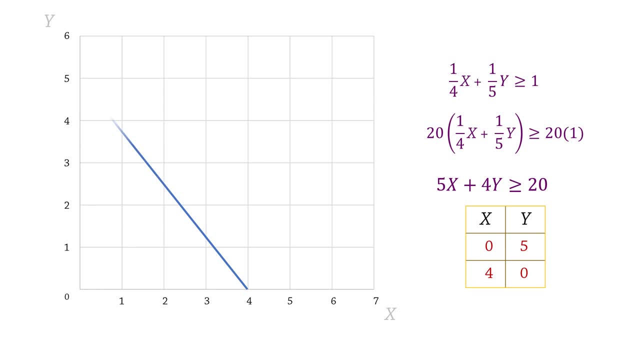 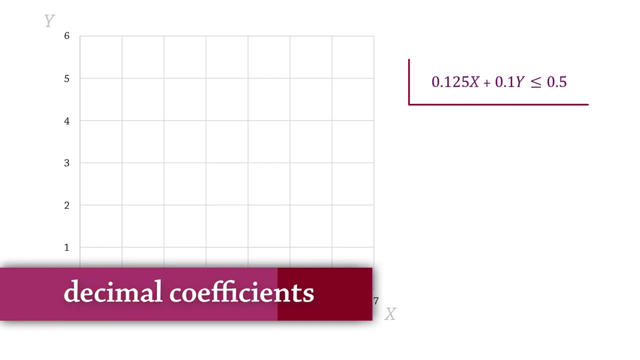 5x plus 4y greater or equal to 20, which, as we saw earlier, is satisfied above the line here. And if we have decimals as shown in this inequality, we can also first clear the decimals by multiplying both sides by multiples of 10, based on the number of decimal places we have Since the maximum we 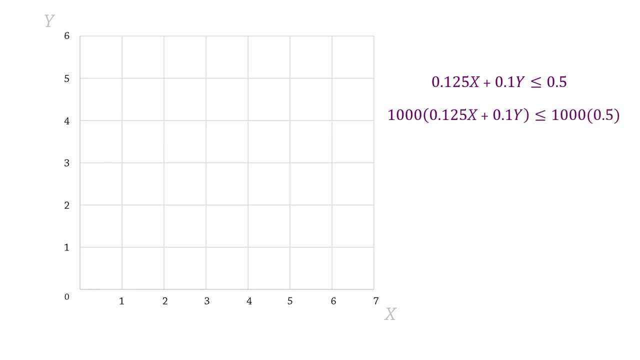 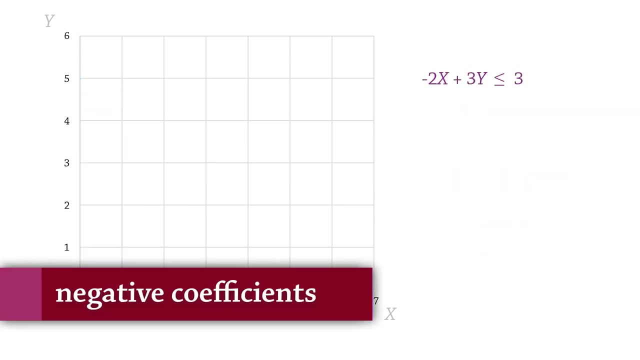 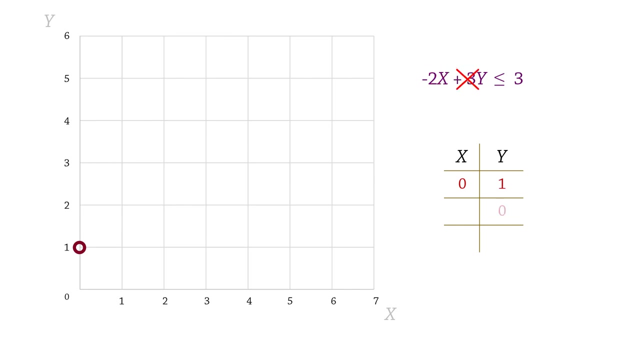 have here is 3 decimal places. we can first multiply both sides by 1000. And if we now divide both sides by 25, we have this initial inequality which is satisfied below the line here. Now consider this constraint with negative coefficient. When x is 0,, y is 1.. When y is 0,. 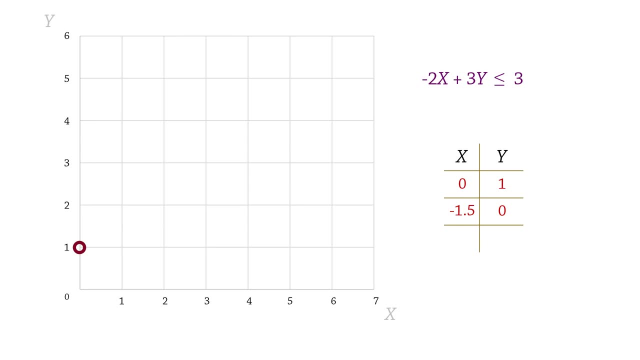 x is negative 1.5.. This second point can be plotted somewhere to the left here, but I'm just going to find another point that does not involve a negative value. This is because sometimes the negative value is too far away and using it makes the feasible region appear too small. 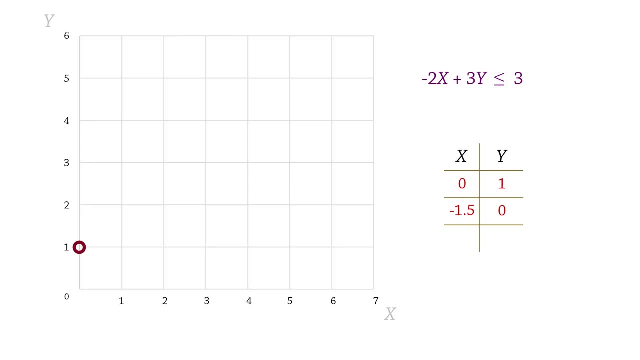 So I'm going to find another point that will fall into this quadrant. I will pick a value for x or for y, whichever is more convenient, and calculate the other. I can rewrite the equation of the corresponding line as: 3y equals 3 plus 2x. 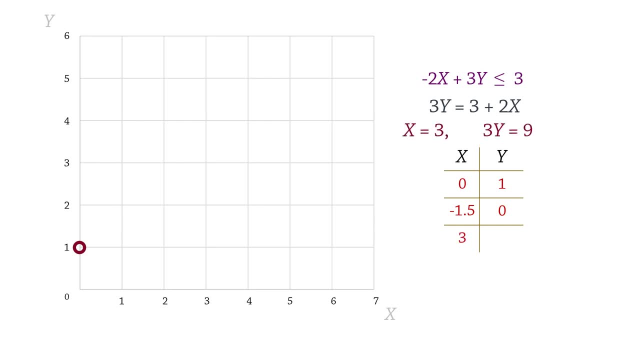 So when x equals 3,, 3y equals 9, and y equals 3.. And here is the equality line for the constraint. To determine the satisfying the constraint, I will pick a point on either side of the line to be sure. 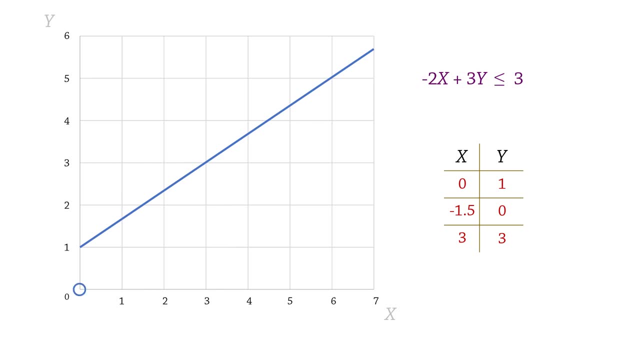 The origin 00 is always an easy one to use When both x and y are 0,. the left side of the inequality is 0,, which is less than 3.. So the inequality is satisfied in that direction. Note that if I pick a point on the other side, for example 03,, I obtain 9 on the left, which is not. 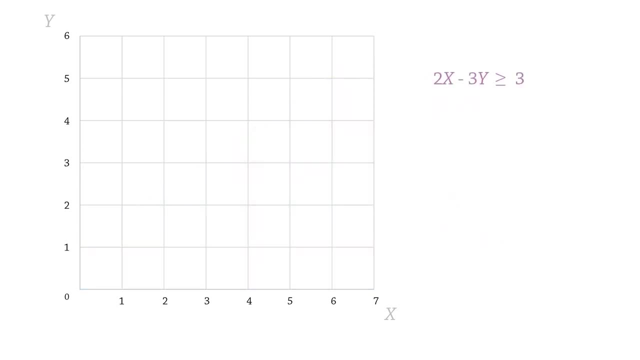 less or equal to 3.. Now suppose we have the inequality: 2x minus 3y greater or equal to 3.. When y is 0, x is 1.5, and when x is 0, y is negative 1.. 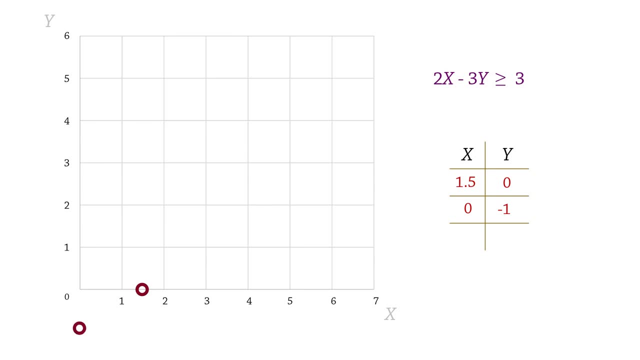 0, negative 1 can be plotted down here somewhere, but again I'm going to find a positive value. I can rewrite the equation of the corresponding line as: 2x equals 3 plus 3y. Thus, for example: 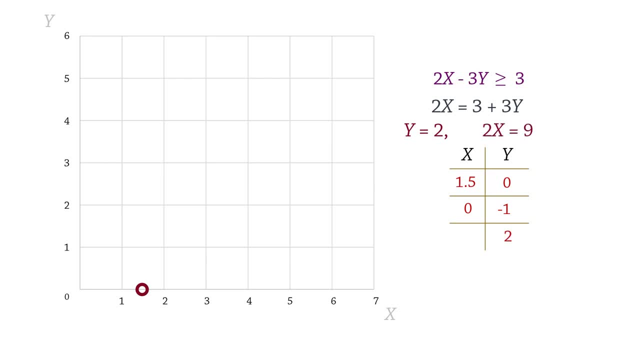 when y equals 2,, 2x equals 9, so that x equals 4.5.. Here is the equality line. Testing the constraint at the origin, we see that 0 is not greater or equal to 3.. So the inequality is not satisfied in that direction. But 0 here gives us 8. on the left: